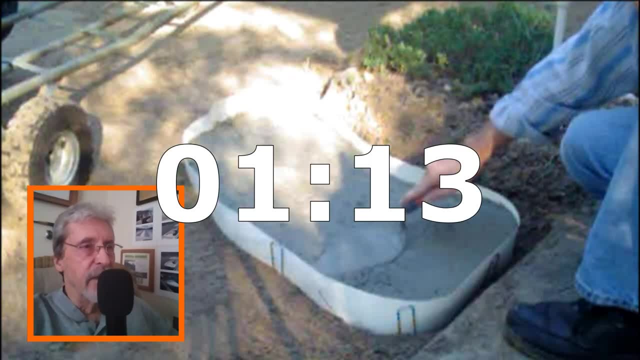 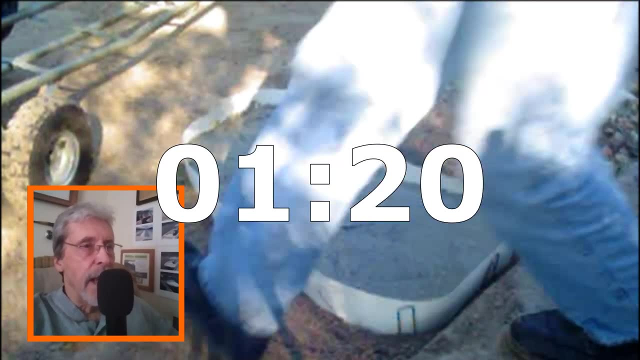 moist and you can mix it right in the form. here I am now leveling all the way up to the top of my concrete. I'm just going to pour my out the surface, making it nice and smooth. start tapping the surface. that helps bring the water to the surface and that makes it nice and smooth. if you 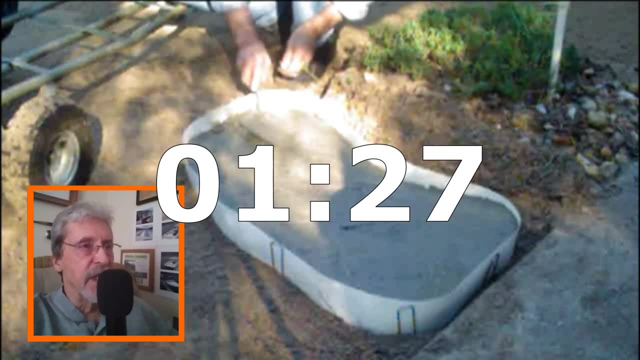 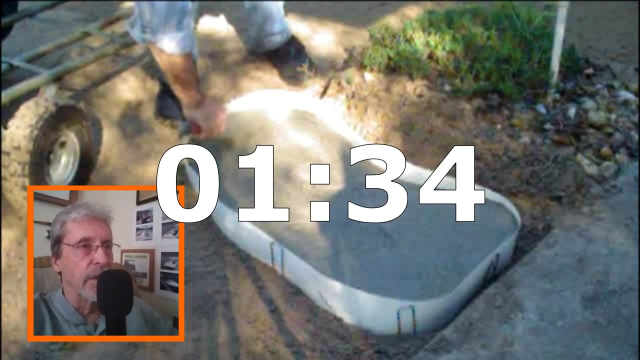 don't do this, you're gonna have a rough stone. so the more you work the surface, the smoother it's gonna get. and this is the time to you when you want to start adding your colors and you can blend your colors into the surface of the stone. I like using two or three colors when I do my stones. all right, that's. 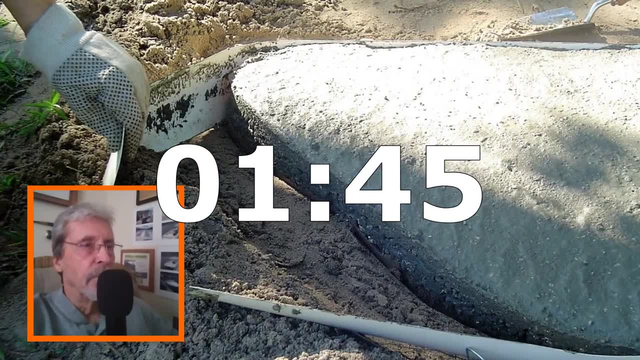 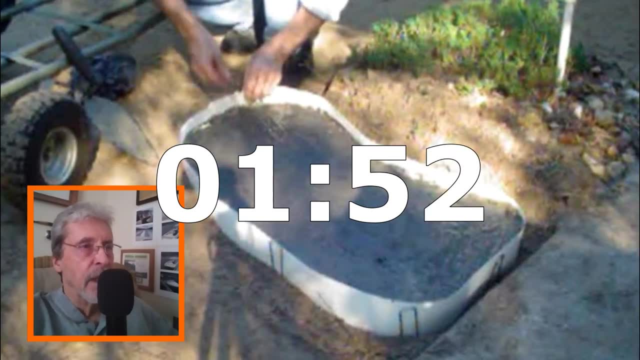 looking pretty good. I like that. alright, now it's time to remove the form. I'll do this gently, you'll have no problems, and if you do, you can always fix it right here I am removing the anchor pin- don't know what pin. right here I want to. 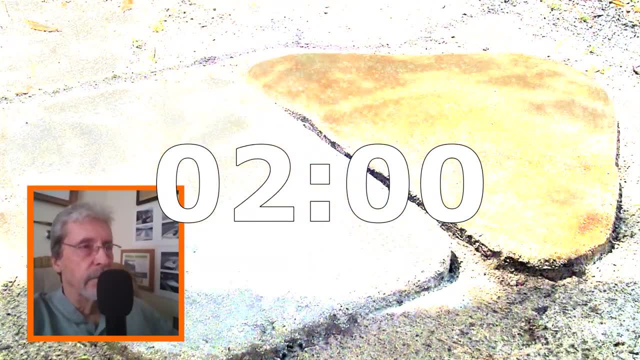 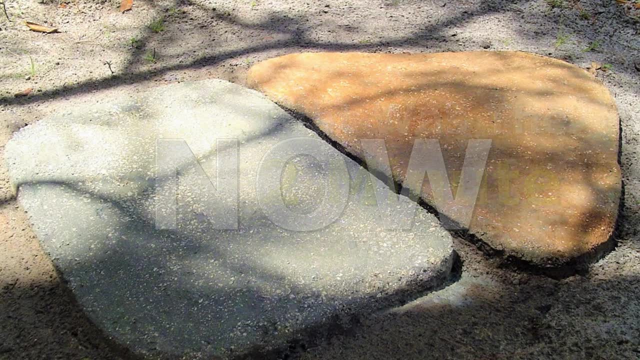 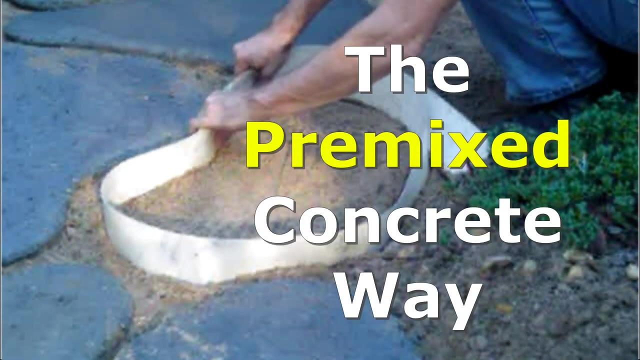 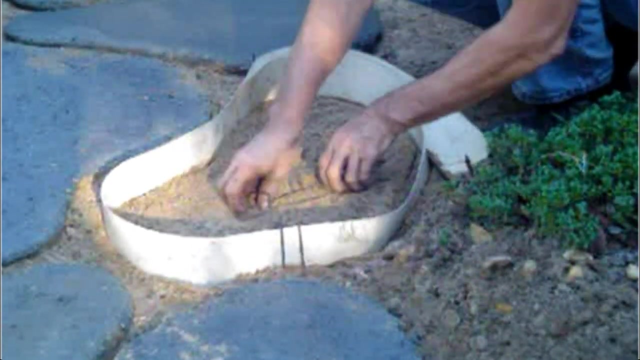 remove. all right, just give a little jiggle, they'll loosen right up and there you go and you're done. now I would like to show you another way to make stones. you the pre-mixed way, putting my anchor pins in, holding the form to the shape that I'm looking for. 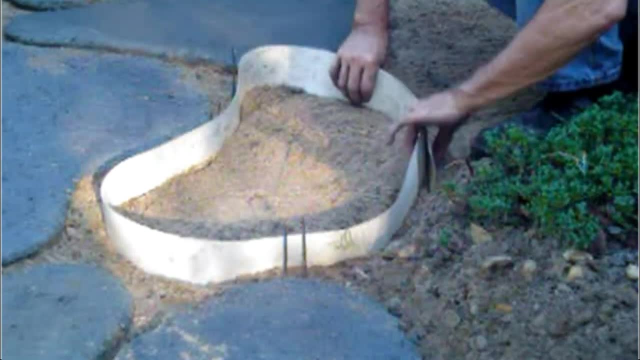 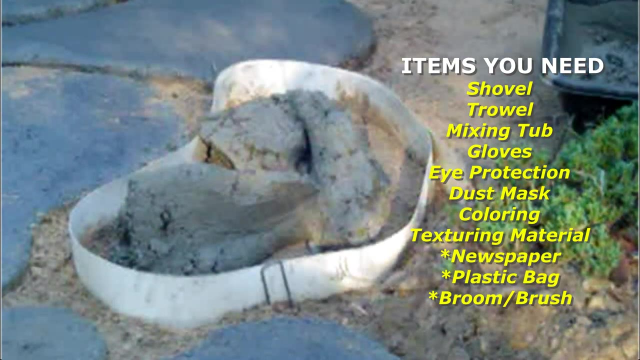 now you can make any shape and size you want. this is the size I'm using right now. here's some of the items that you'll be needing now. here's my pre-mixed concrete, which I am going to be using right now. I'm going to be using this. 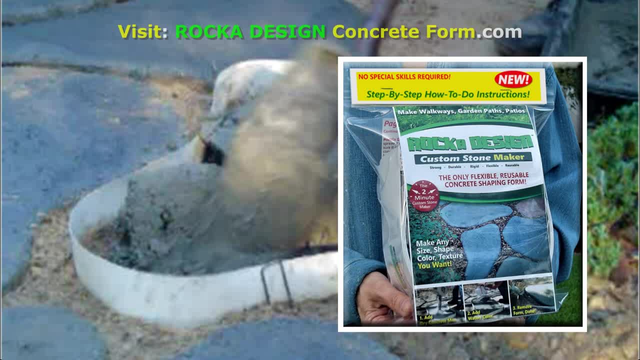 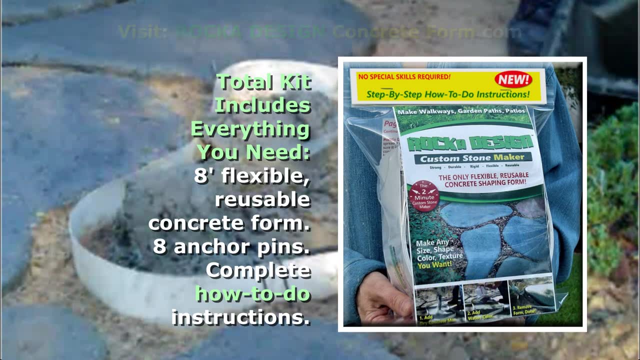 which I mixed in a tub over there. now I'm putting it right into this form, and it does look like I'm using a lot of concrete in this form. that's because there's something I want to show you, so I'm putting it all into this form. 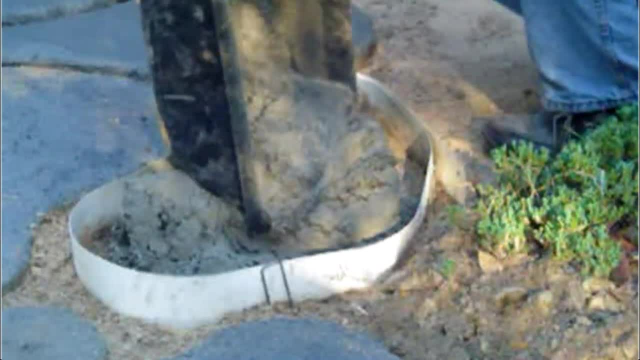 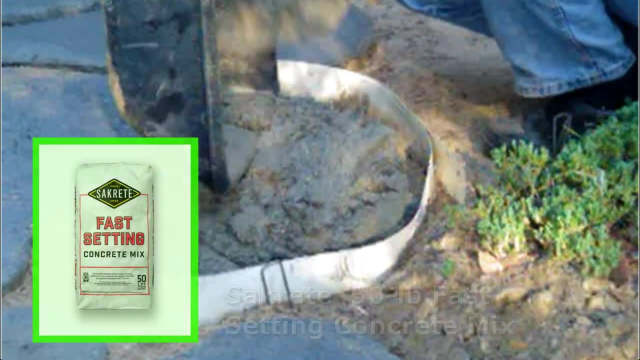 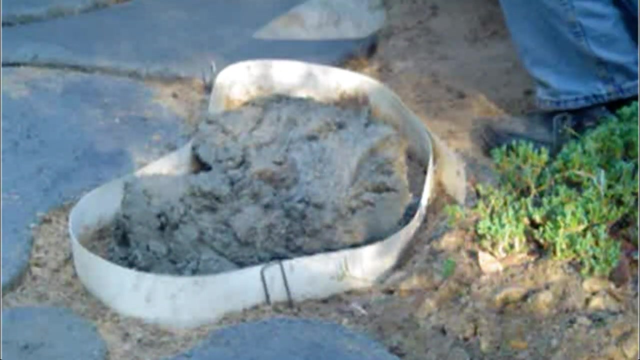 trying to get it all out of that tub there. all right, I don't want anything getting hard in that tub, so I'm scraping it all out. really, I'm putting a lot of concrete in there now. I like using the sacrete 50 pound fast setting concrete. 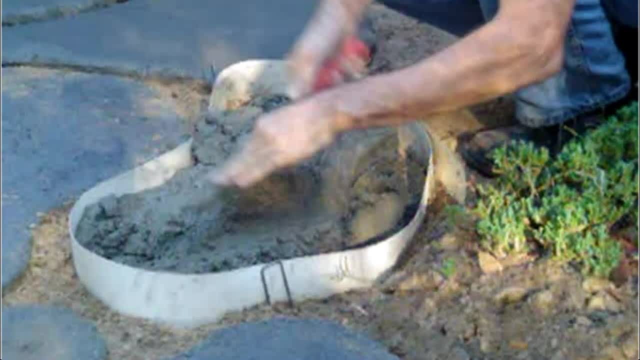 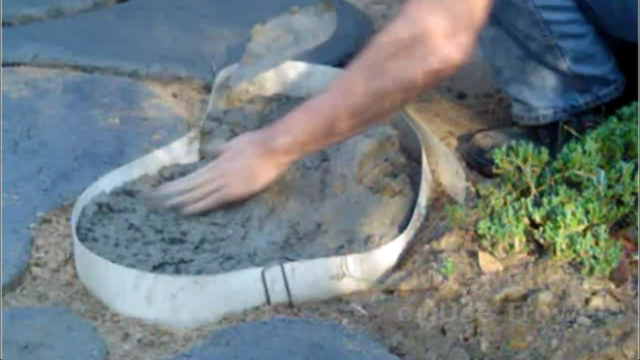 mix. a 50 pound bag is nice- you can put two bags in this form here- but 50 pounds is a lot easier to carry than an 80 pound bag. now I'm just moving the concrete around now. what I want to do is this. what I 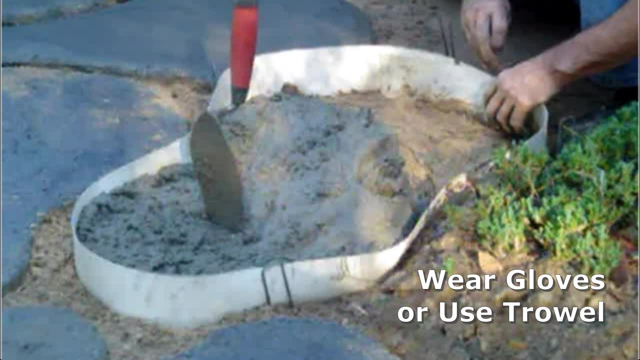 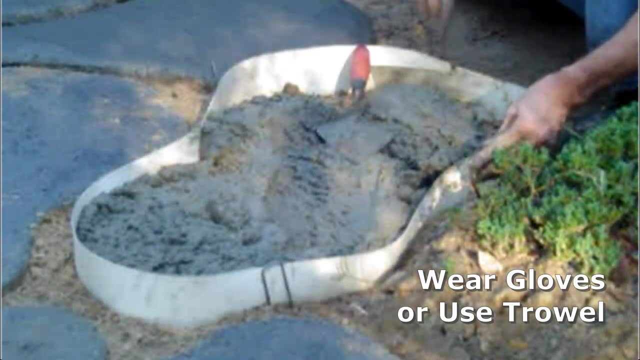 want to show you, even though you started the project, you can still open the form and make changes, putting my anchor pin in there to hold the form. now I'm spreading out the concrete there. I need an anchor pin right there. there we go. now we're all set. now you can. 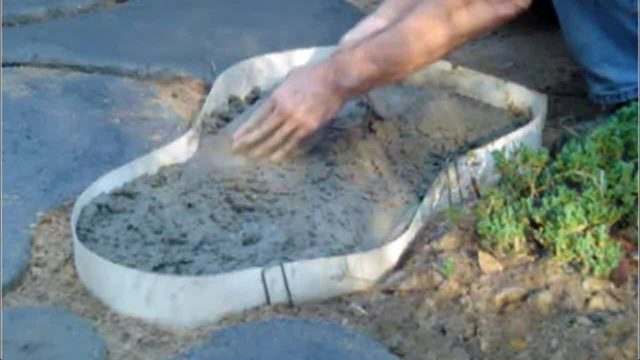 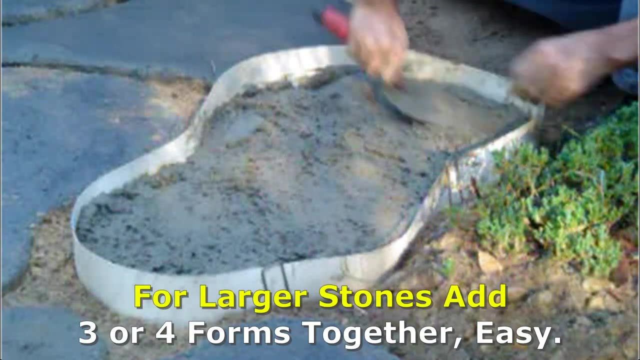 see how the anchor pin holds the form in place. just moving the concrete around. that's all I'm doing. now you want to make sure that the concrete is the same. the stone here is the same height as all the other stones. you don't want one stone higher than the other, so that's all I'm doing. 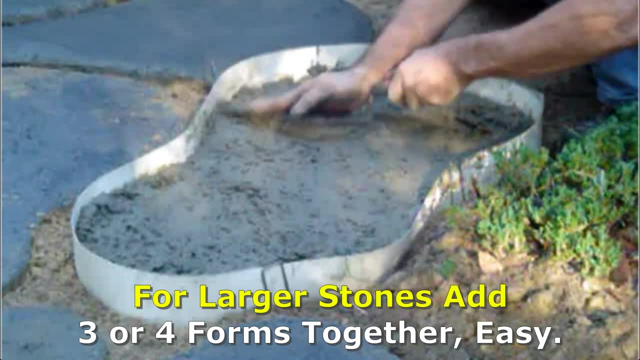 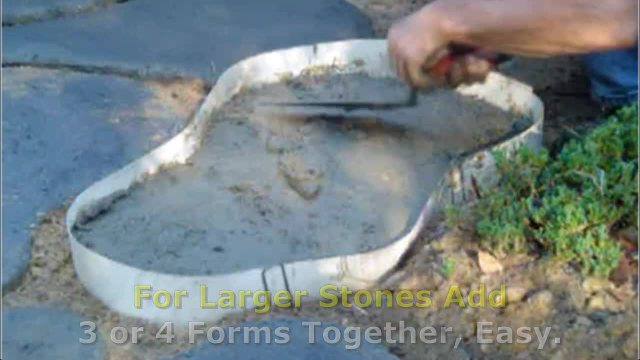 right now it's just moving the concrete around, leveling it all out, and you can see: by moving the concrete around and working the surface, you can see that that's starting to get more wet. the moisture is coming to the surface. now, if you need, you can always add more water because you want a. 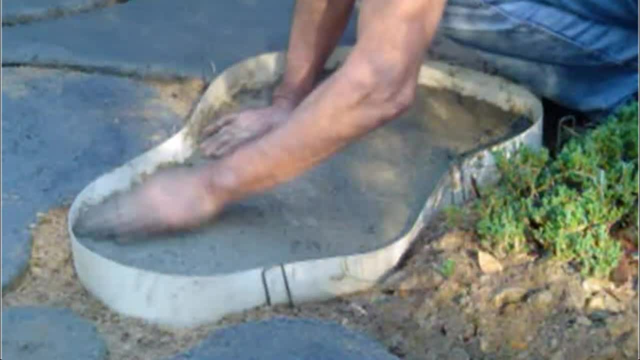 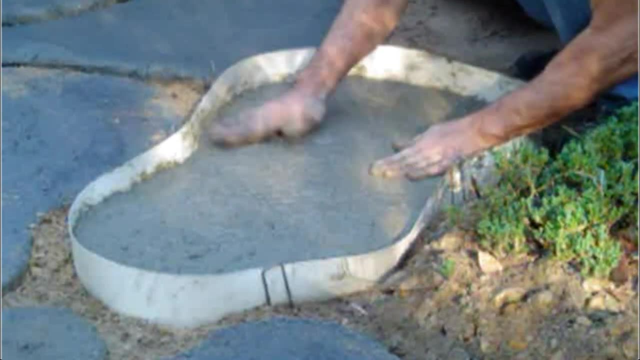 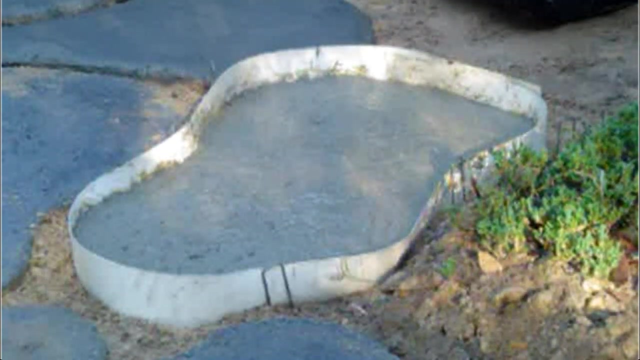 nice wet surface. now, tapping the surface like this- this is what you want to do. tapping the surface brings the moisture to the surface. this is what makes the top of the stone smooth. if you don't do this, you're gonna have a rough stone. you don't want that, so just keep tapping it and that's what. 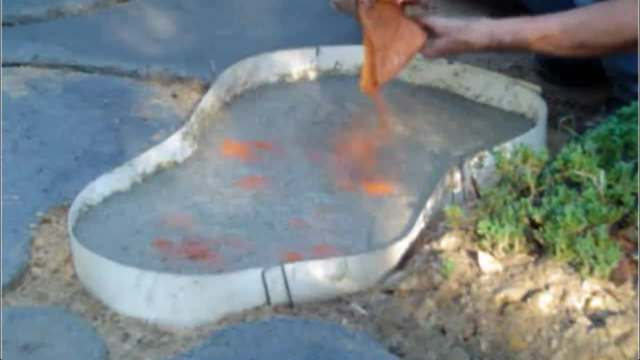 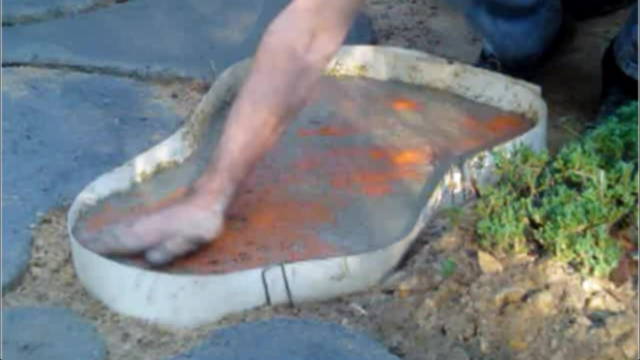 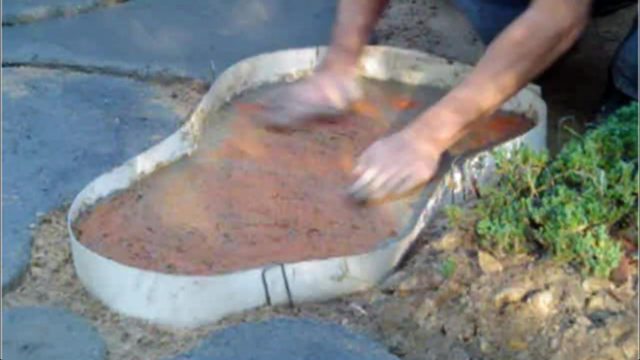 you want when you start adding your color here. I am now adding my color. now I'm just doing the surface color. I'm going down about a half inch into the stone. there's no need to go through the whole stone, not unless you plan on breaking the stone in half. so I'm just doing the top half inch layer of the stone, rubbing it in. 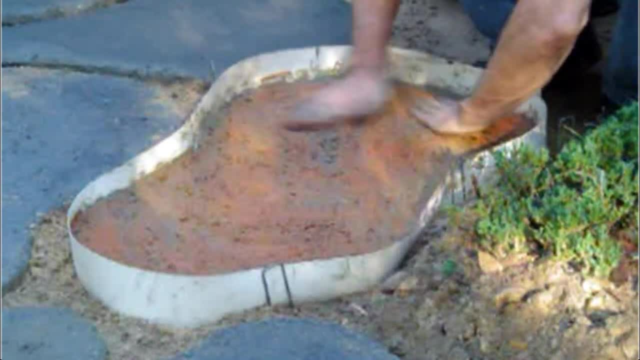 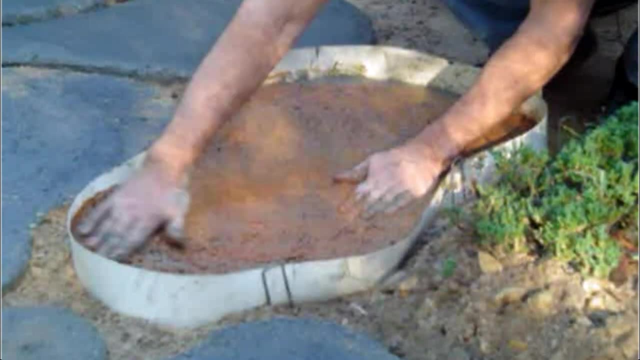 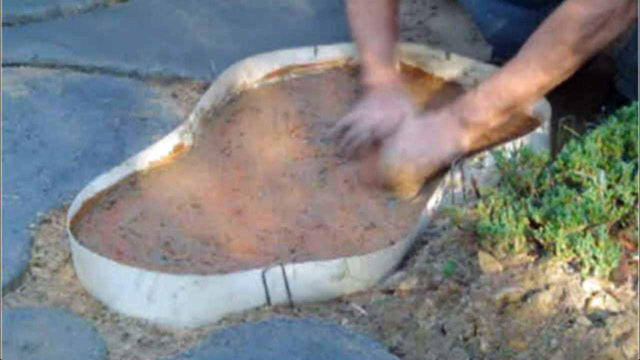 mix it in good, and by doing that again I'm still bringing moisture to the surface, which helps with that coloring. now I like using two or three different colors, because real stones have multiple colors, so I'm just working it in, getting into the edges there, the corners. it's looking good. 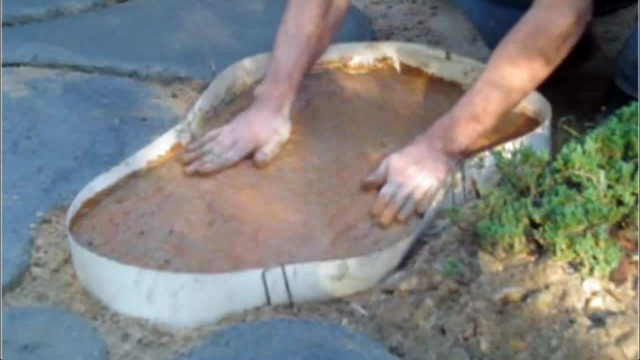 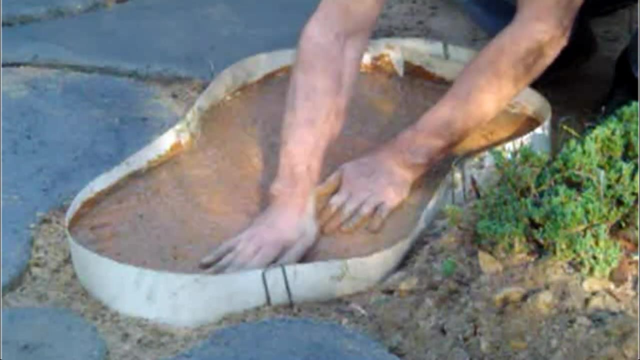 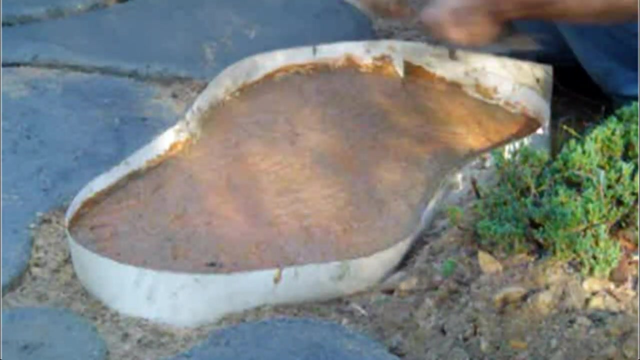 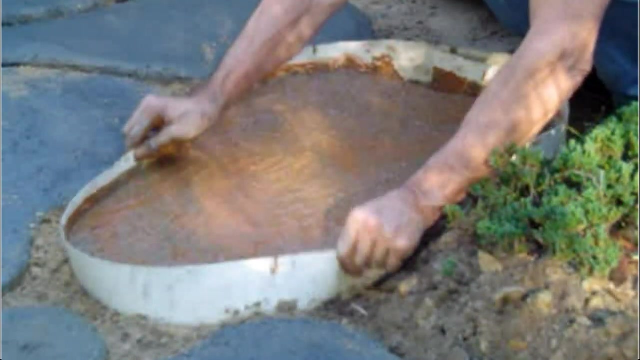 just patting it down. now don't, uh, do use bare hands, use gloves, don't do what i'm doing. or use your trowel, move it around. all right, now i'm going to remove the form. i'm taking out my anchor pins. now you just be gentle, no problem. just a little shake there, a little jiggle, there's the shake.